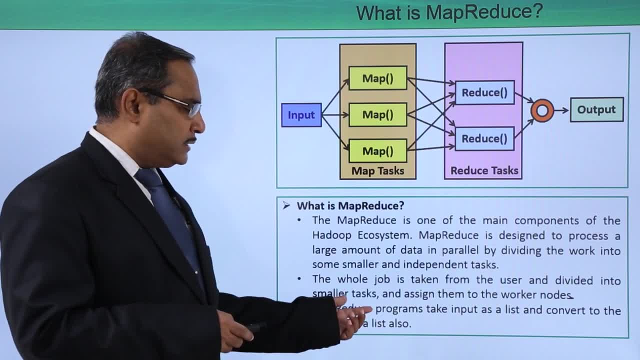 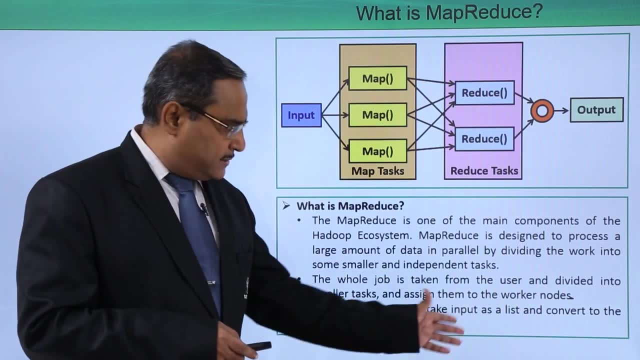 Det\' 길974 per cent of our Avatars Issued mass is brain- has been executed when the setup isning up by Microsoft URL job is taken from the user and divided into smaller tasks and assign them to the working nodes. Map-produced programs take inputs as a list and convert to the output, also as a. 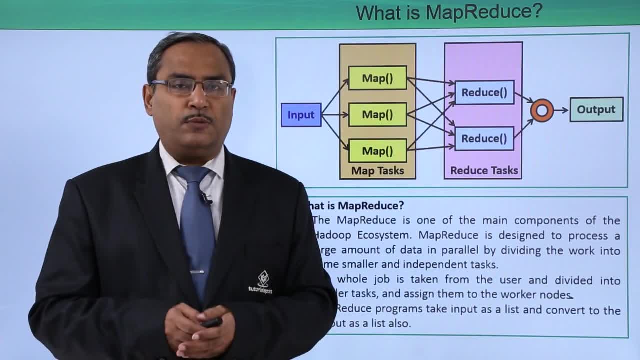 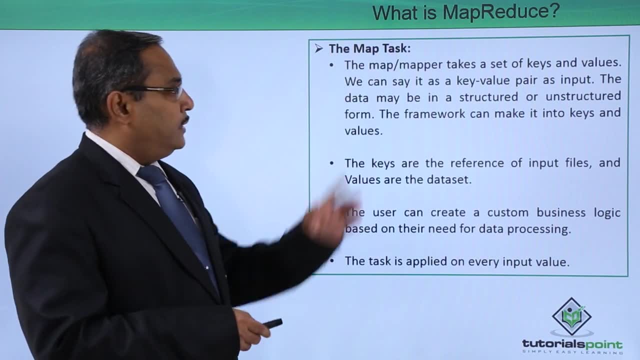 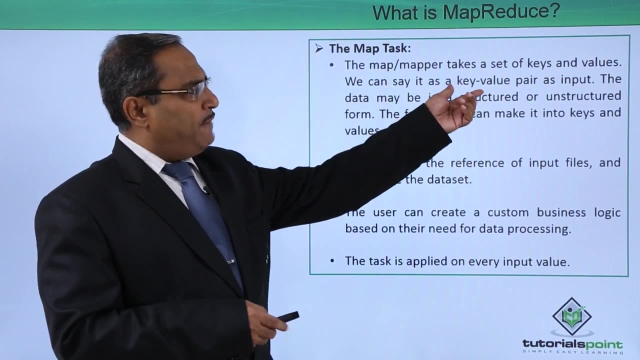 list. So it will take the input as a list and it also converts output in the form of a list. So let us go for some further criterias. The map or the mapper tasks a set of keys and values. we can say that it is as a key value pair as input. So this particular data 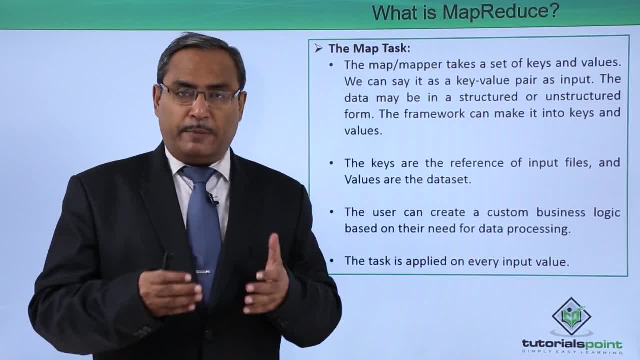 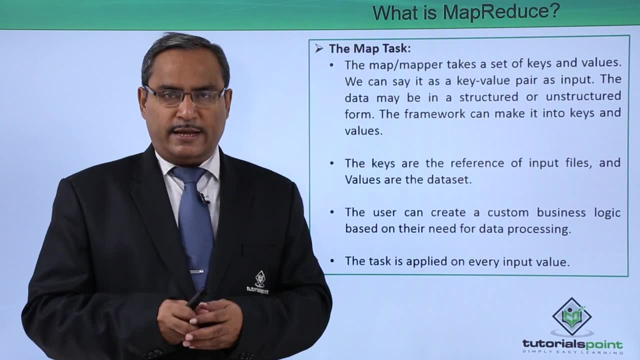 will be in the form of key value pairs. Now questions might be coming in mind that what is key and what is the value. So key is actually nothing but a reference to our data set, and values are nothing but the data sets. So key can be treated as a reference to a data. 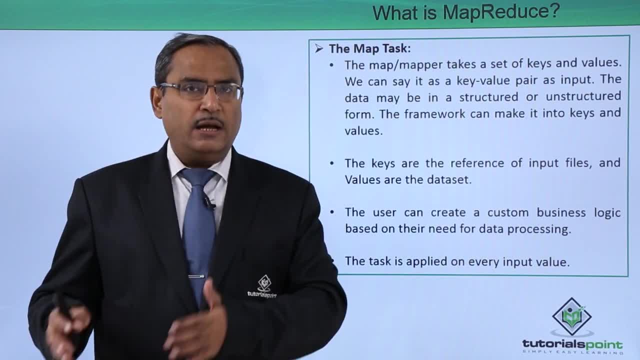 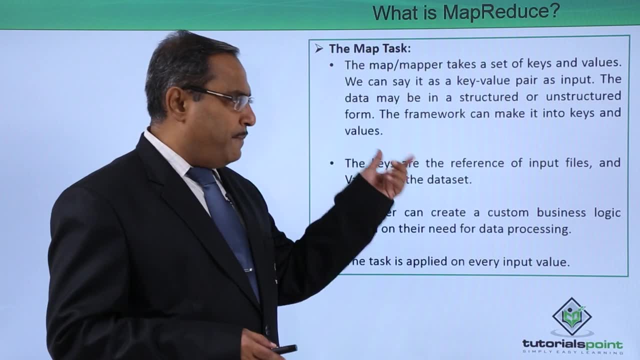 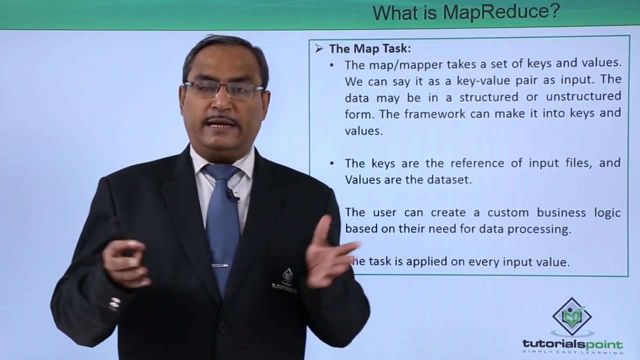 set or reference to a file and the value is nothing but our data set. The data may be in Structured or unstructured form, and the framework can make it into keys and values. So the data set may be in the structured. that means in the form of, say, database and database tables. 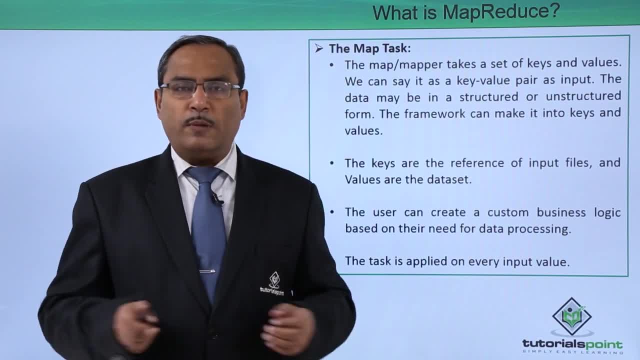 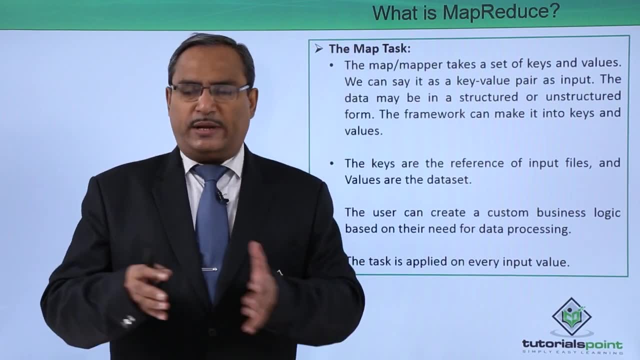 where the data can be divided or can be represented in the form of rows and columns, and unstructured midware will be going for text files, PDFs. we are having the images, we are having the videos, and they will be known as the unstructured data. The framework can make it into keys. 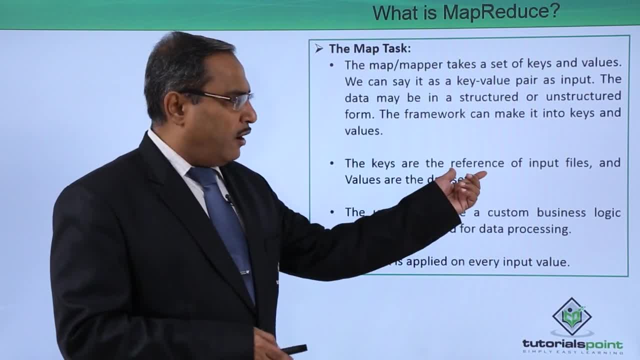 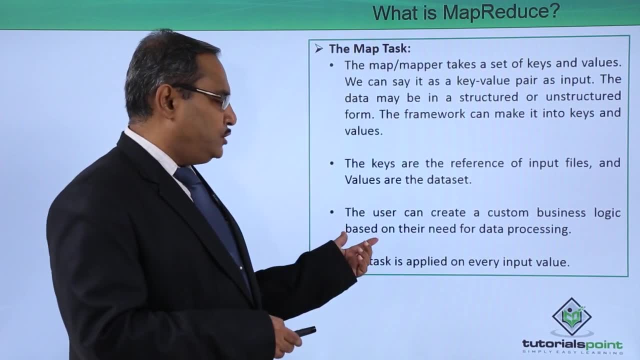 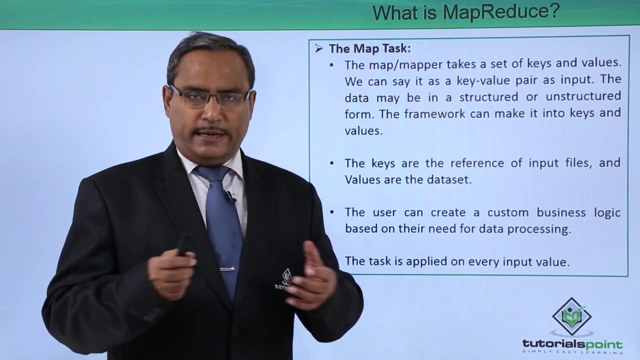 and values. The key are the reference of input files, and values are the data sets. The user can create a custom business logic based on the need for the data processing. So what kind of processing will be done? that can be customized depending upon the business need. 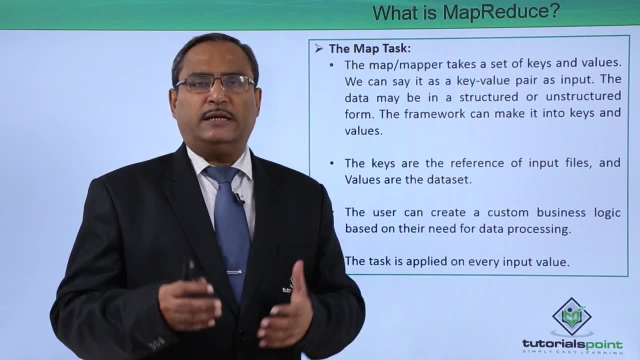 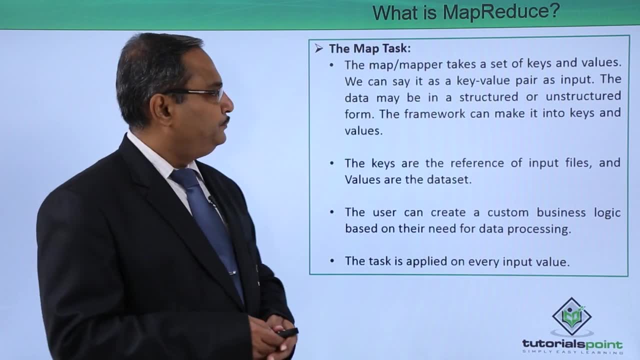 the respective operations will be carried out. the respective processing will be carried out on the data set. The task is applied on every input value, So the data set can be created on every input value. Now we are going for the reduce task. The reducer takes: 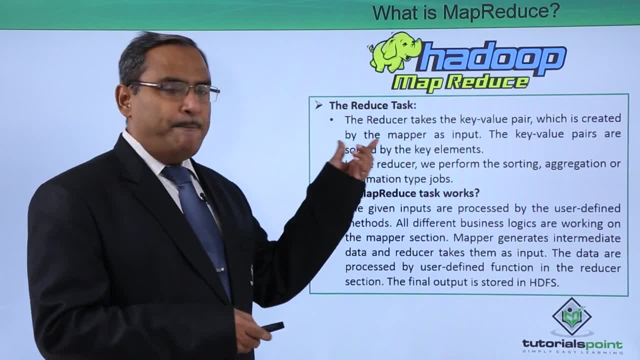 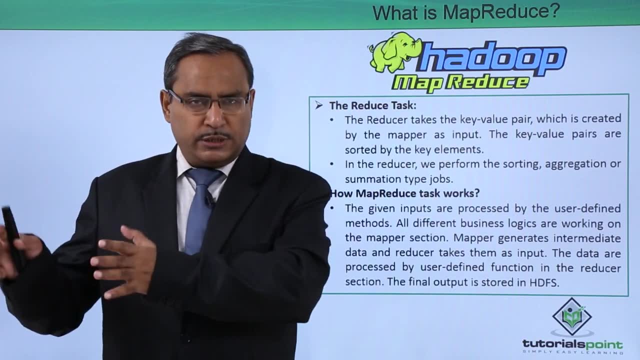 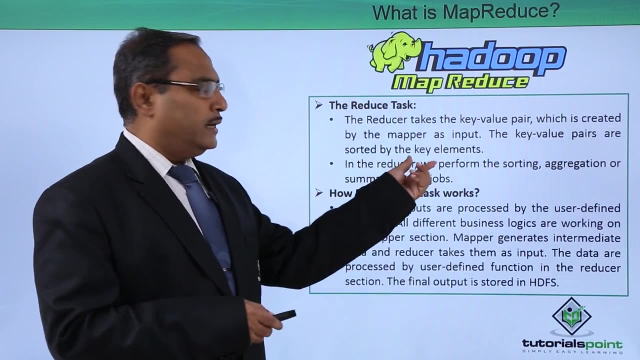 the key value pair which it which is created by the mapper as input. So mapper is taking the input and mappers output will be the input to the reducer and reducer will produce the respective output. accordingly, The key value pairs are shorted by the key elements in case. 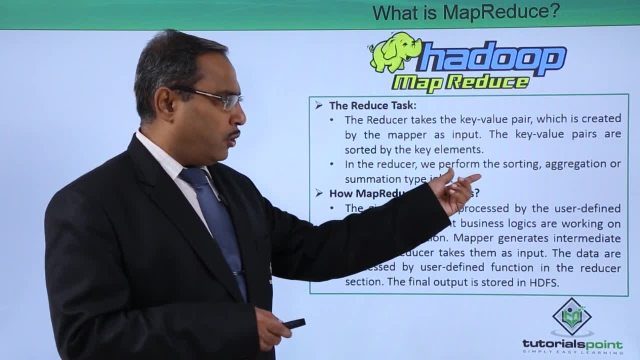 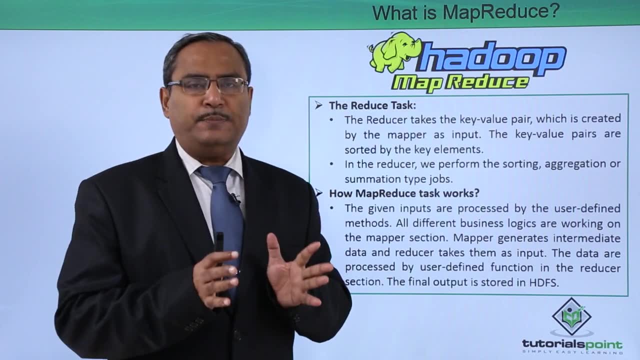 of reducer And in the reducer we perform the shorting, aggregation or summarization type of jobs. That means here we are going for some aggregation type of job. We can go for, say, submission, we can go for, say, counting, we can go for 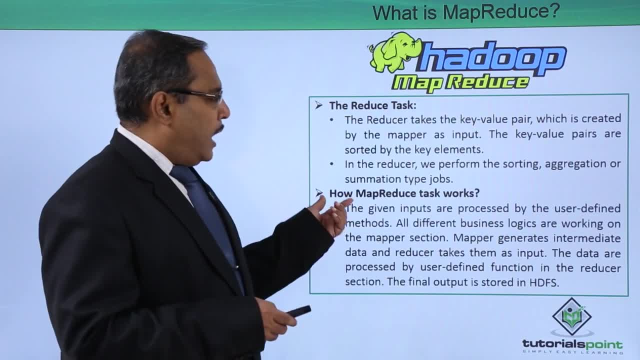 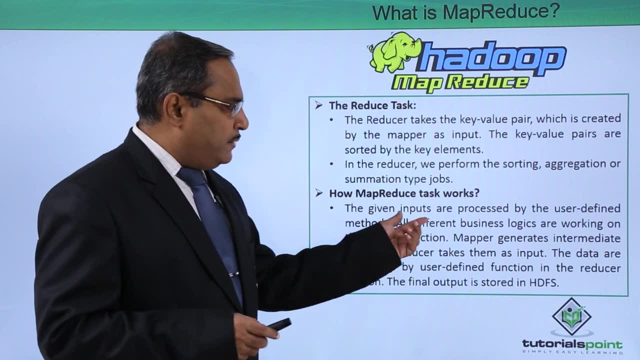 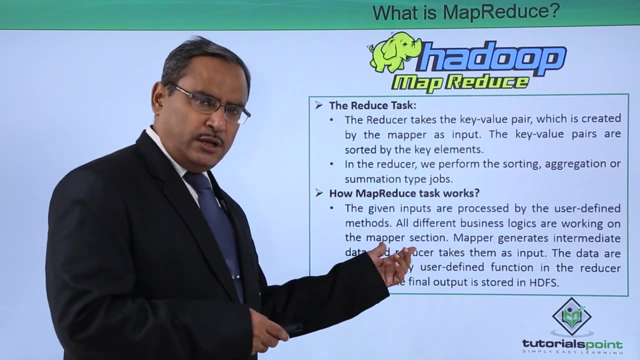 say maximum, minimum calculations and so on. How map reduce task works. So now let us go for the macro view of the system. The given inputs are processed by the user defined methods. all different business logics are working on the mapper section. So business logic. 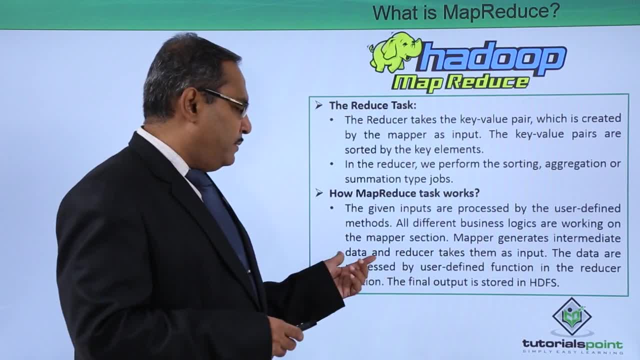 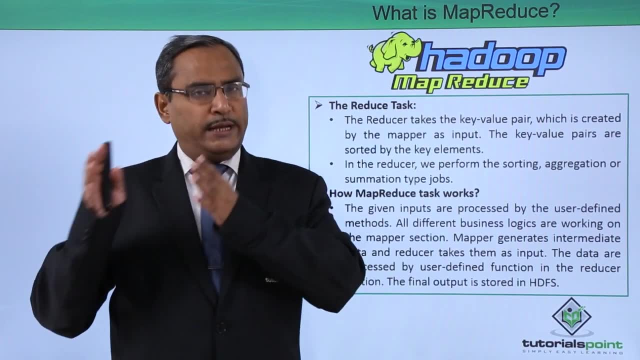 will be working at the mapper section and the mapper generates intermediate data and reducers takes them as input. as i told you earlier that the output of the mapper will be the input to the respective reducer, the data are processed by the user. different function in the reducer section. 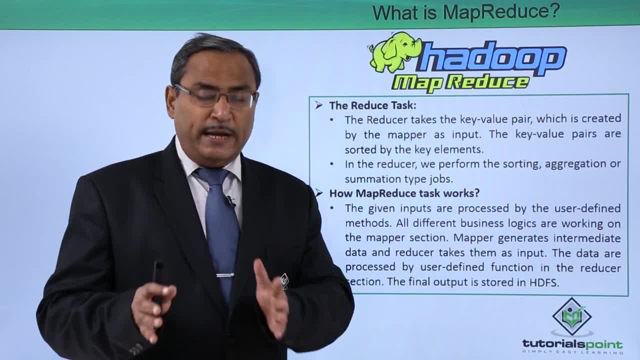 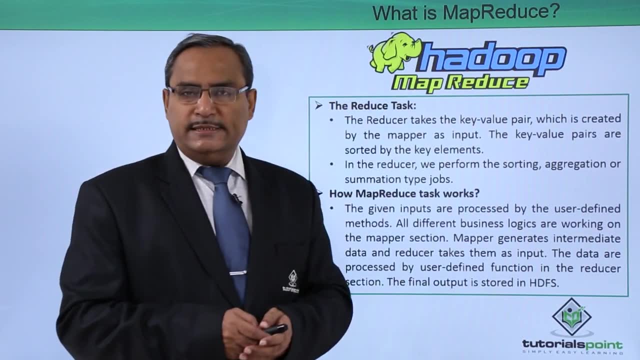 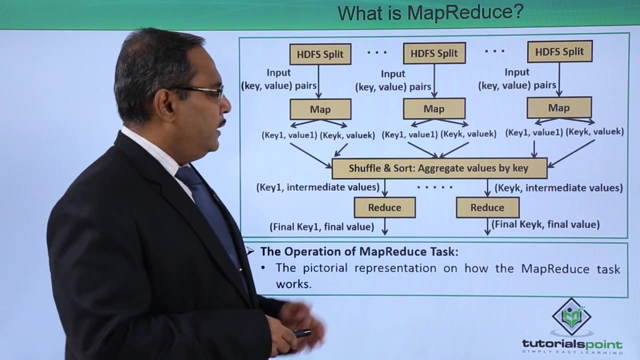 so the data processing will be done at the reducer section, depending upon the business logic, depending upon the user, different function or operation- and the final output is stored in hdfs, that is, hadoop distributed file system, where the final result will be stored there. now let us go. 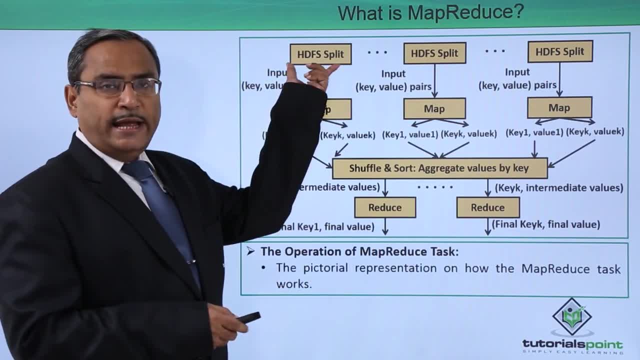 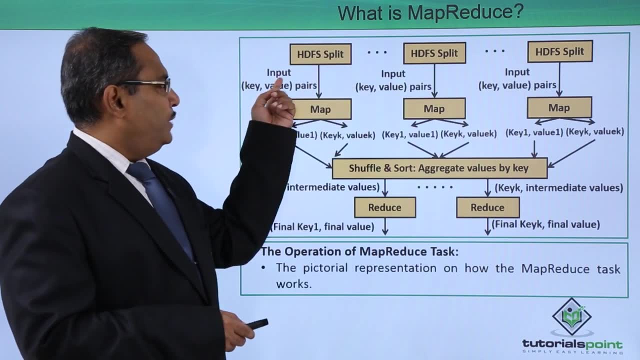 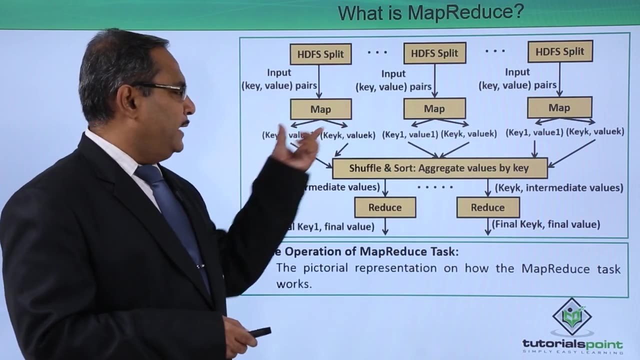 through one proper diagram here. so you are having here hdfs split, so multiple splits are there. so hadoop, distributed file system split will be there. so input will be key value pairs. in this way it will be, the input will be obtained to the respective mappers. so now, here the mapping is. 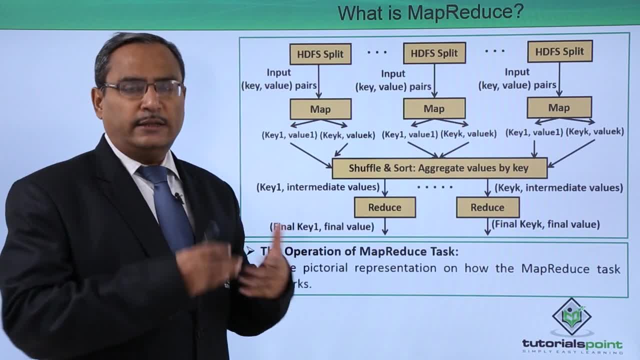 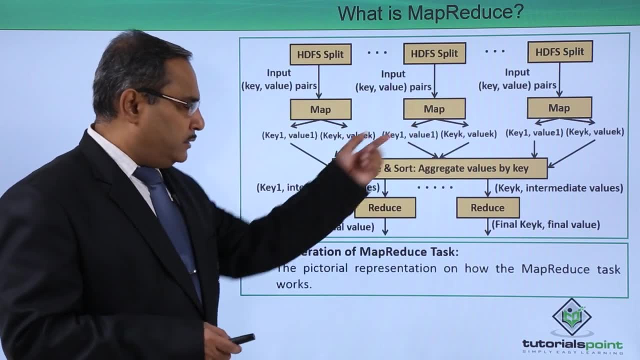 taking place and it will be now. it will be dealing with multiple keys and the respective value. so q1 value of the mapper is the input value of the mapper and the input value of the mapper is the value one, two key, k to value k. in this way the mapper will be working now. their outputs will. 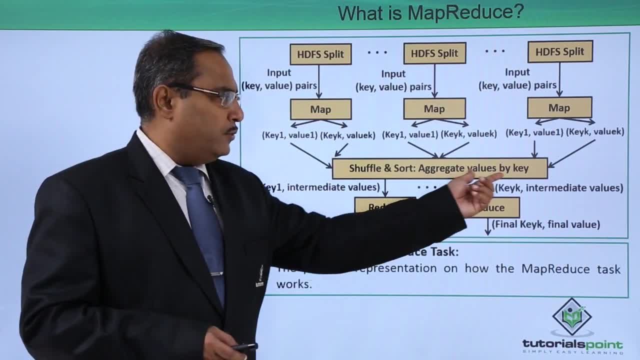 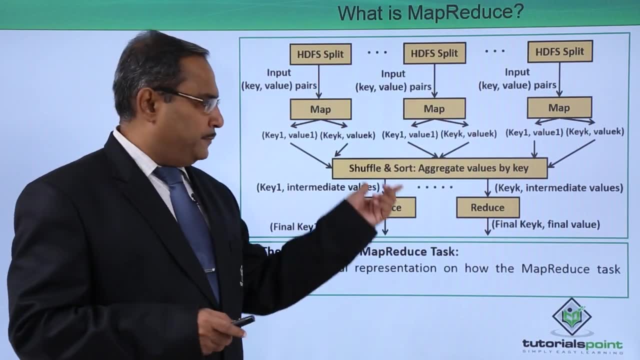 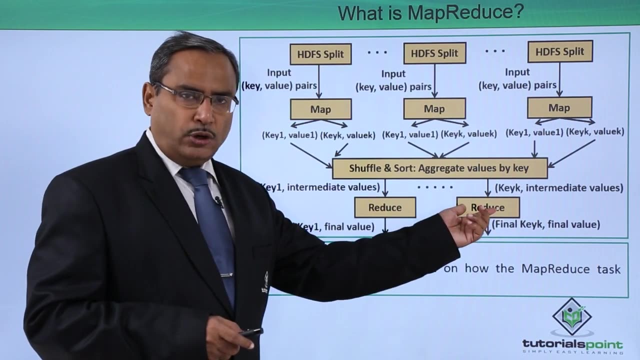 be coming to this shuffle and short. so here they aggregate values by the key, so depending upon the same key, so they will get aggregated, then the result will be obtained. that means the output of this shuffle and shot operation will be obtained to the reducer. so these are the reduced methods. 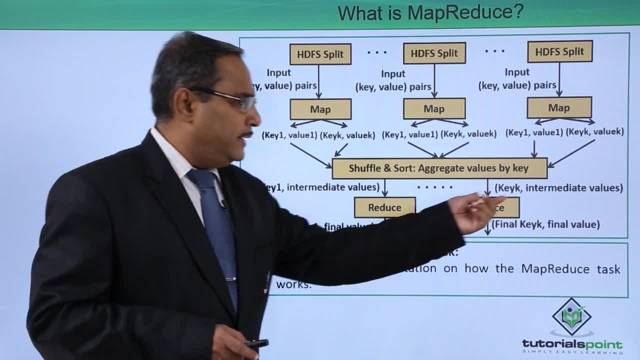 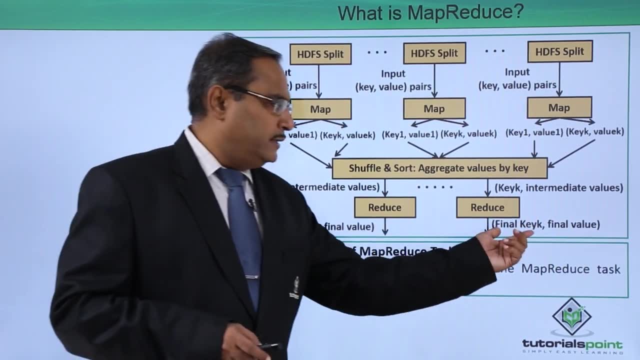 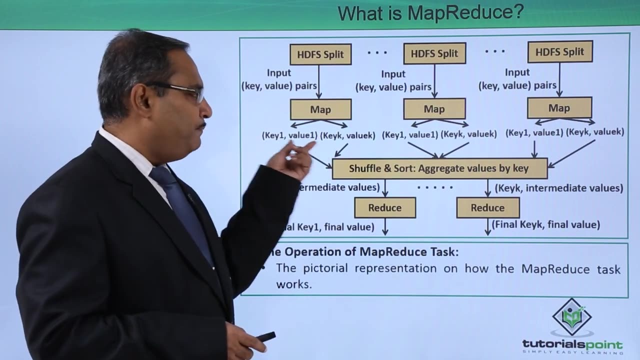 are working here. so we are having the q1 intermediate values and then key k intermediate values will be coming to the respective reducers and then final key 1 and final value and final key k and final value will be obtained in this way. So initially we are having this key 1 value 1, key k value k. in this way we are having 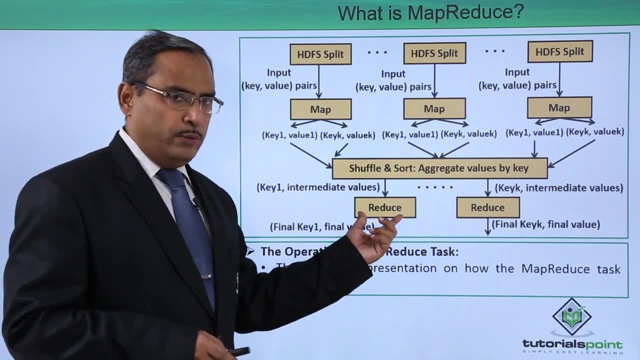 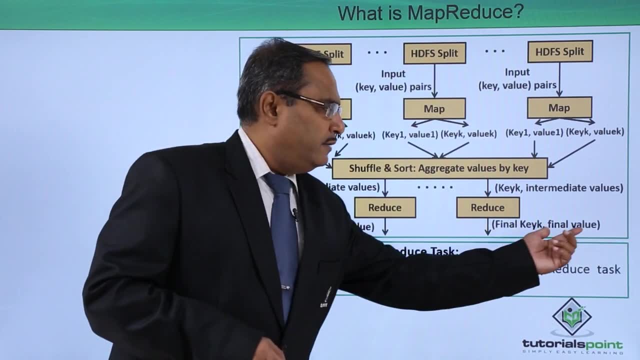 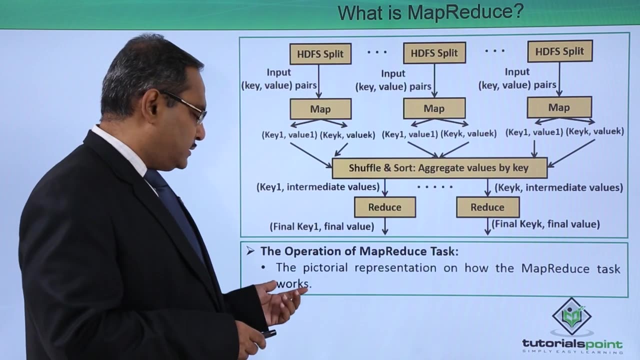 then here we are having this shuffle and shot, then the reduce method will be working on it, then we are finally getting final key 1 value, final key k, then final value. in this way the things will be obtained as output. The pictorial representation on how the map reduce task works. we have shown that one in 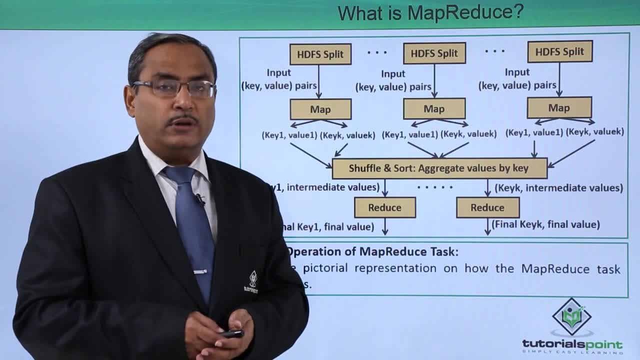 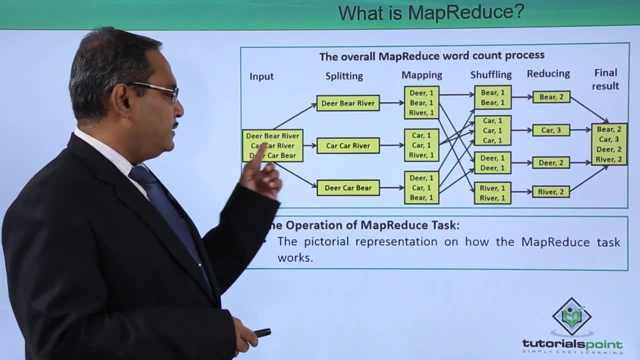 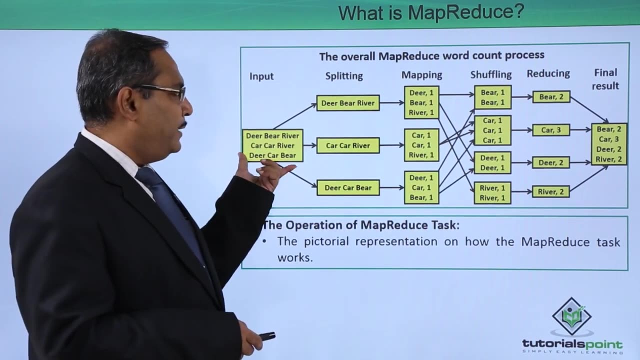 this diagram. So let us go for another elaborative example for the better understanding. So here we are having one example here. So deer beer river, car car river, deer car beer. So these are the value sets we are having. so set of values we are having. 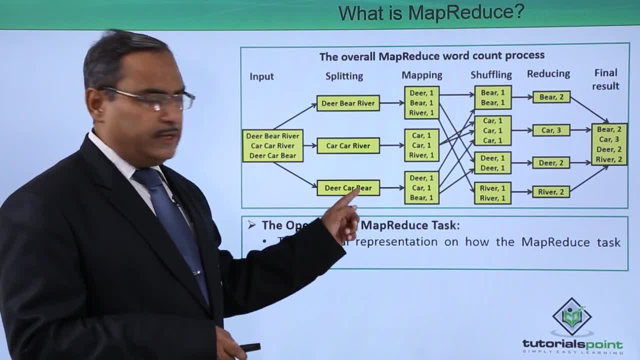 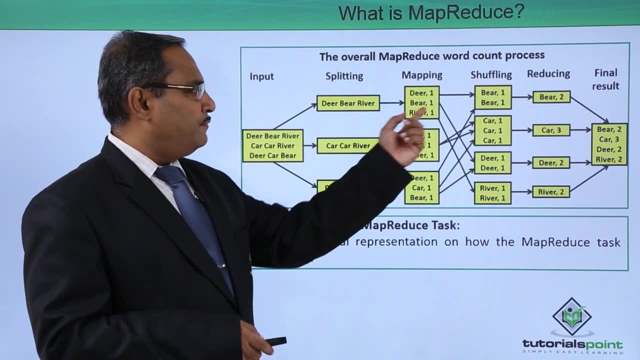 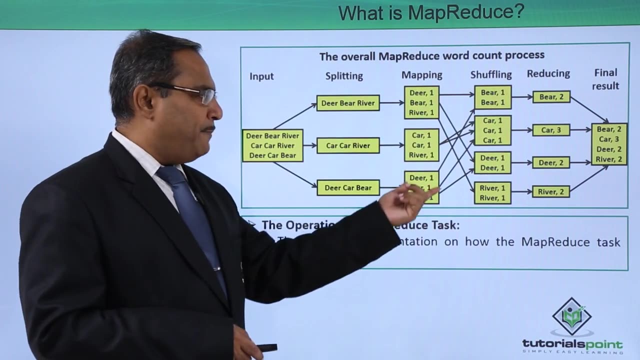 So now they will be splitted. in this way, the splitting has been done, Now the mapper is there, So here the mapping is taking place. So I am finding deer for one count, beer for count 1 and river for count 1.. Car for count 1, car for count 1 and river for count 1. in this way the mapping is taking. 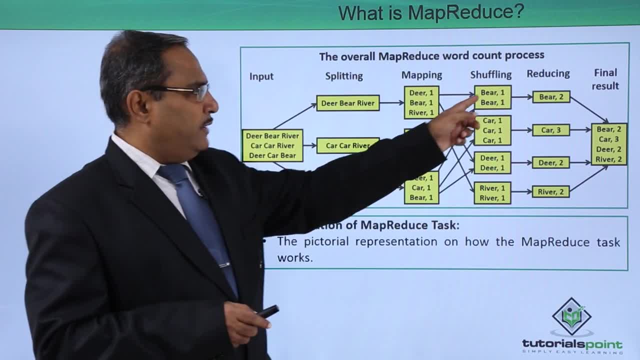 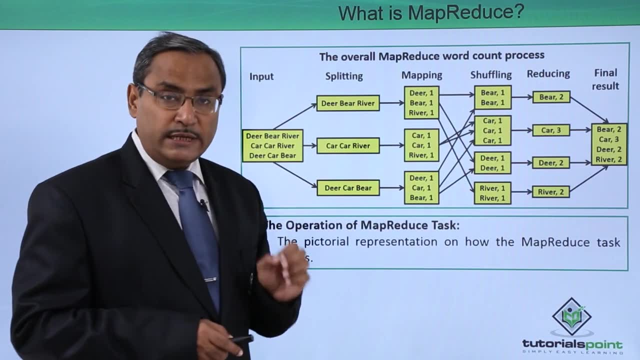 place. here we are having this shuffling and shotting, So here you can find we are having this beer. only the beer keys are there. only the car keys are there. only the deer keys are there, only the river keys are there. Then here we are going for the reducing. 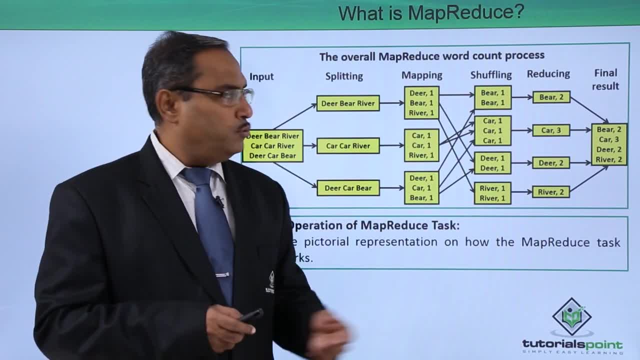 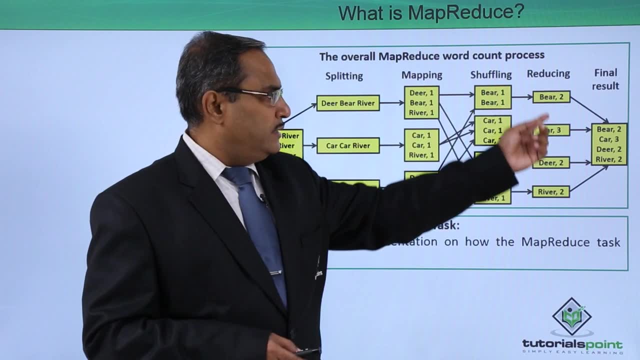 So this beer has occurred for 2.. So here the aggregation method is: is count actually. So here car has occurred for 3 times, deer has occurred for 2 times and river has occurred for 2 times. So here this is my reducer, which is doing the reducing. 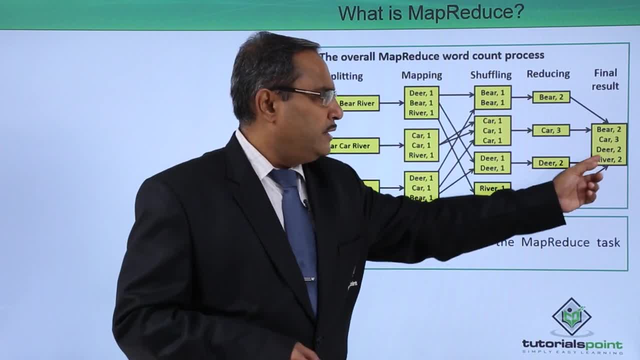 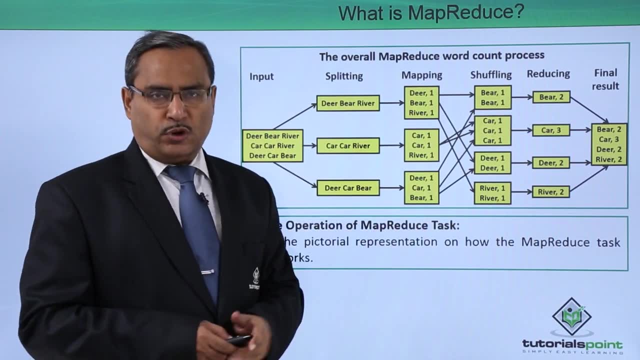 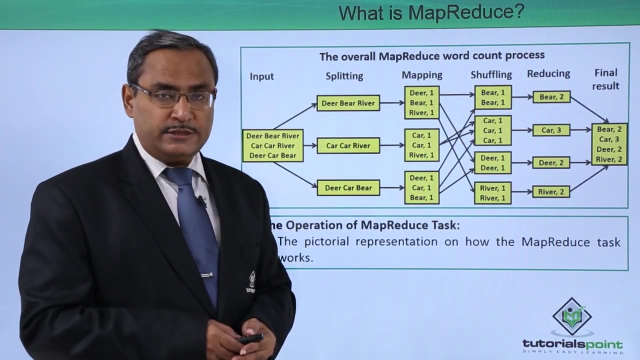 and here we are having this final result that is, beer 2, car 3, deer 2 and river 2.. So here you can find that how the overall map reduce what count process is getting executed into multiple different phases. So this example is a very interesting one, and also it is 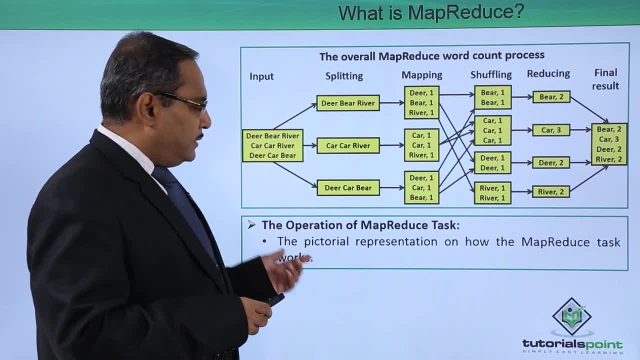 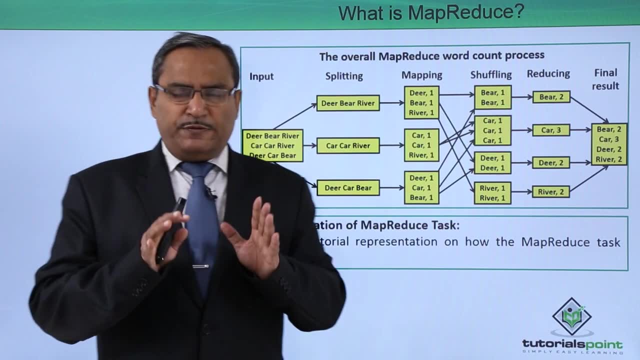 clear our doubts and it is clear our conception. also The pictorial representation on how the map reduce task works. we have shown that one in this way. So in this video we have got the idea that is what is map reduce. Thanks for watching this video.